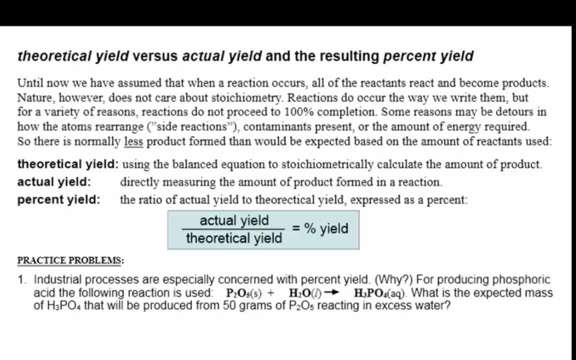 So we're getting a lot of practice with stoichiometry here, and that is the name of the game. There's a lot of applications with stoichiometry in chemistry. We're going to be using it a lot in different ways, And so practice is very important to get these basic calculation structures into your head so that when we apply it in different directions, the basic stoichiometry won't get in the way. You really need to get this into your head. 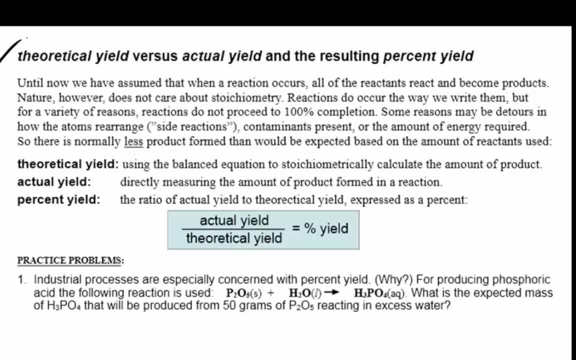 So so we have had some practice with theoretical yield and actual yield and resulting percent yield already, But let's go a little bit further into that. So until now, we've assumed that when a reaction occurs, all of the reactants react and become products. Nature, however, does not care about what we think about how things work. it'll do what it wants. And reactions do occur the way we write them, But for a variety of reasons, reactions do not proceed to 100% complete. 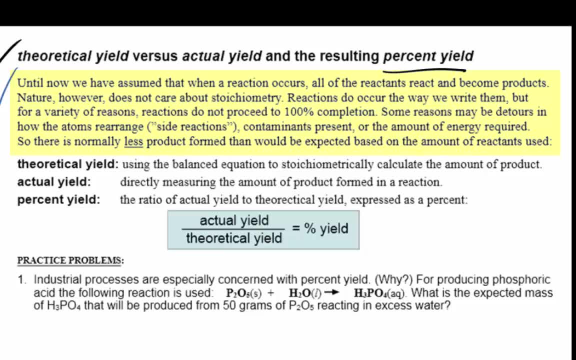 Some reasons may be detours in how the atoms rearrange, And those are called side reactions, Or there could be contaminants present, or the amount of energy required is not right, So there's normally less product form than would be expected based on the amount of reactant used. 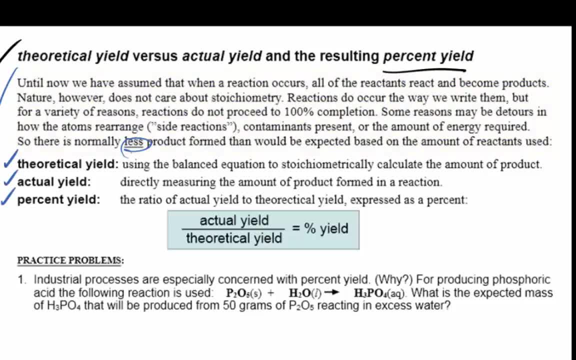 And so definitions which I think we know by now: theoretical yield, using the balanced equation to stoichiometrically calculate the amount of product. actual yield, So the yield is directly measuring the amount of product, And then percent yield is that ratio. 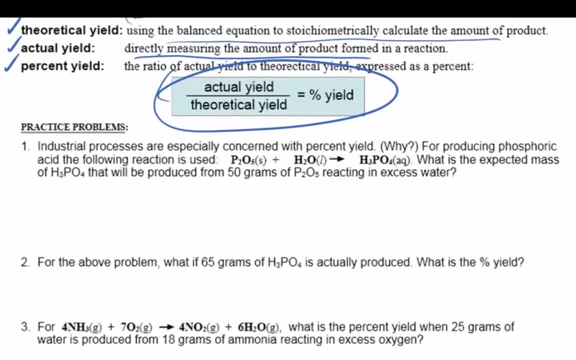 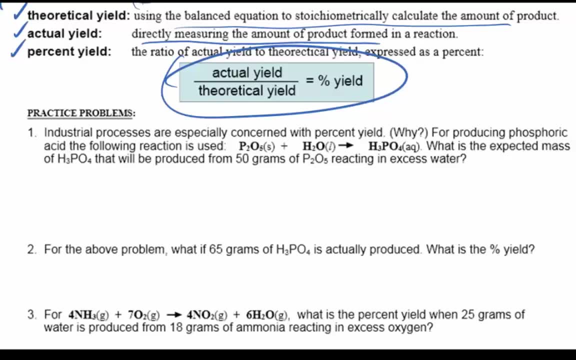 So here's a further application of stoichiometry. We're going to go ahead and go through some of these problems and then you will do a couple on your own. So here we have a problem where P2O5 is reacting with water, making phosphoric acid. 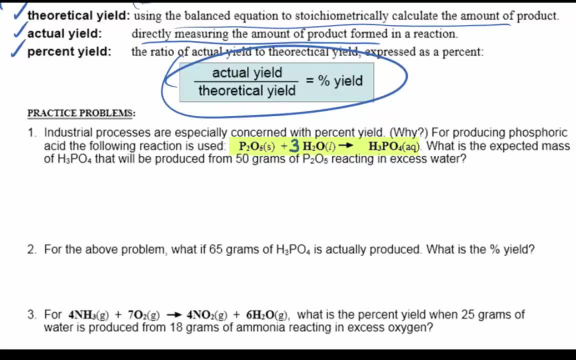 So we need to balance that. If we put a 3 there and a 2 there, I believe that's the right answer. That will do it. So what is the expected mass of H3PO4 that will be produced from 50 grams of P2O5 reacting in excess water? 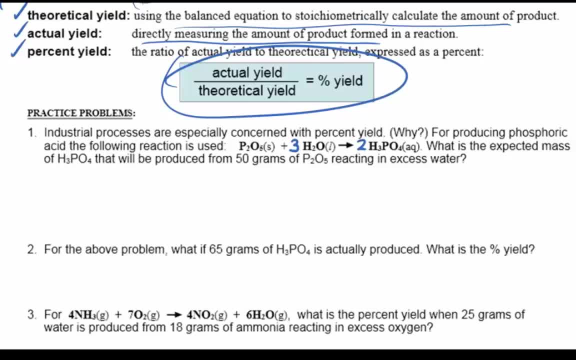 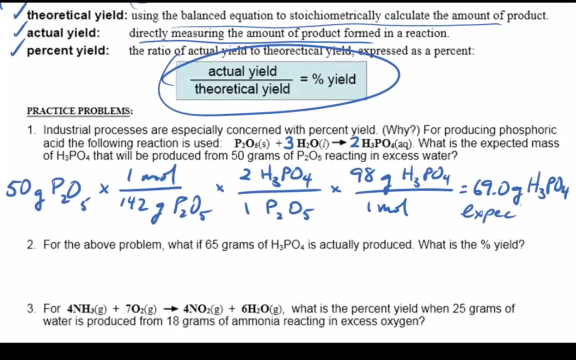 So this is the first step on the way to a percent yield, problem being a basic, straightforward stoichiometry problem. All right, So the expected mass of phosphoric acid from 50 grams of P2O5.. Okay, So here's our theoretical yield, the expected amount. 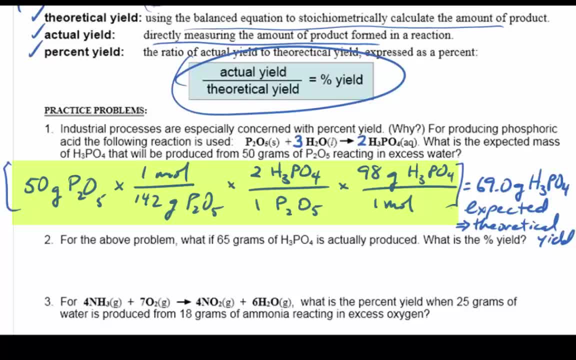 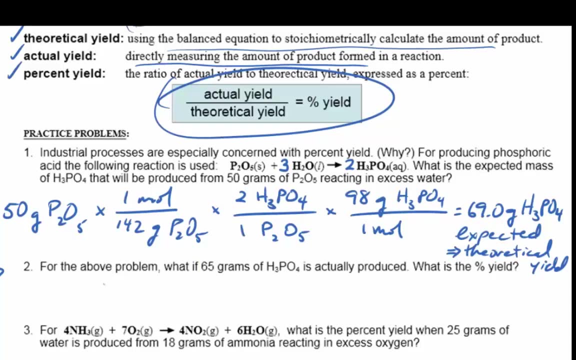 And this was a straightforward mass-to-mass stoichiometry problem. So the second question then takes care of the percent yield part of the problem by giving us an actual yield- 65 grams- And so we simply divide the 65 grams, And so we simply divide the 65 grams. 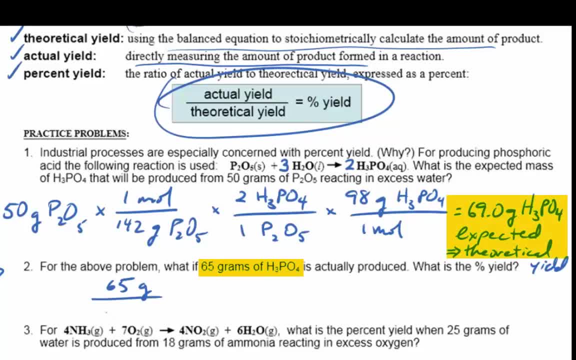 That's the actual divided by the expected amount, 69 grams- And that gives us a 94 percent yield. All right, Let's move on to the next one. So here it's already balanced. I don't know why I did that for you. 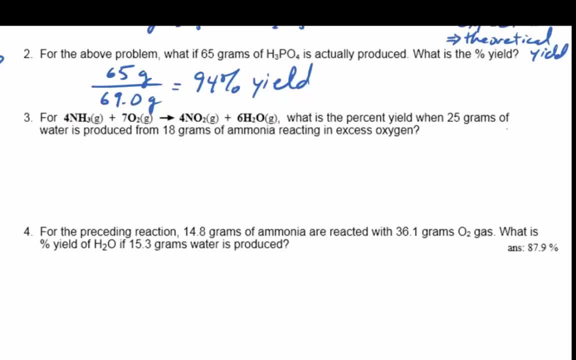 But I guess I did. So. what is the percent yield when 25 grams of water is produced from 18 grams of ammonia reacting in excess oxygen? Here you're given a measured amount. So here's our actual yield, And then you're given a measured amount. 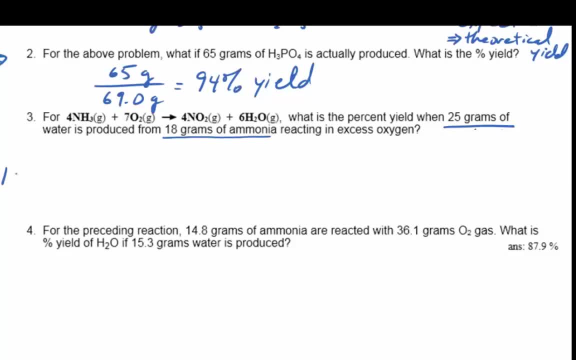 And then you're given the actual amount of ammonia that reacted. So, given that amount of ammonia that reacted, how much water would you expect to be produced? So 18 grams of ammonia, And then our coefficient ratio: water on top and ammonia on bottom. 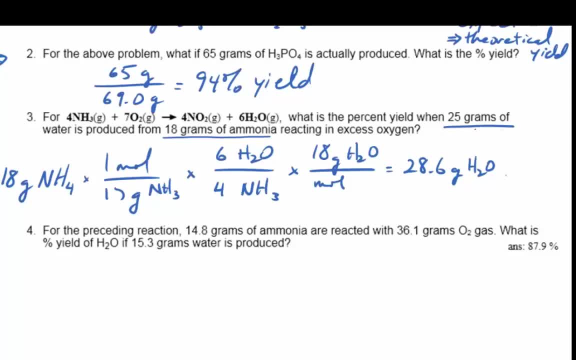 So 28.6 grams of water is the expected amount of water to be produced. So how does that compare to the actual? So we've got 25 actual divided by 28.6 theoretical, And that gives us a grand total of 87.4 percent yield. 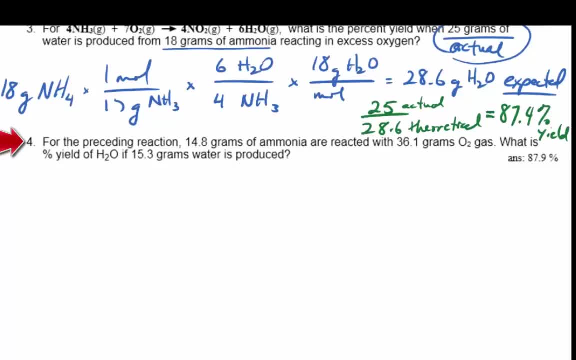 Okay, All right, So for the next one. So here you don't know how much of the water is going to be produced. Here you have an actual amount given in the problem, But you don't know what the expected amount is, because you're given two different amounts of reactant.